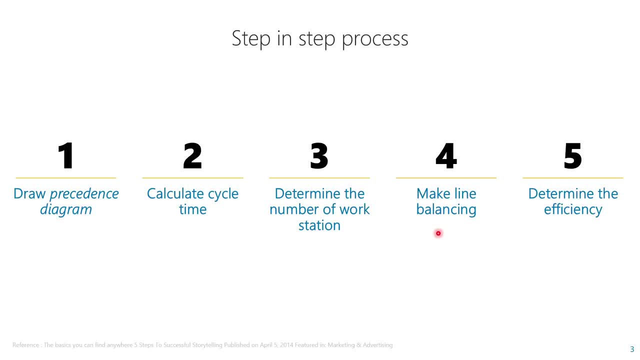 And in the fourth step we have to make line balancing, Determine which process to enter which workstations, And after this step has been done we can determine the efficiency. in the fifth step, To measure either how efficient is our production line is. 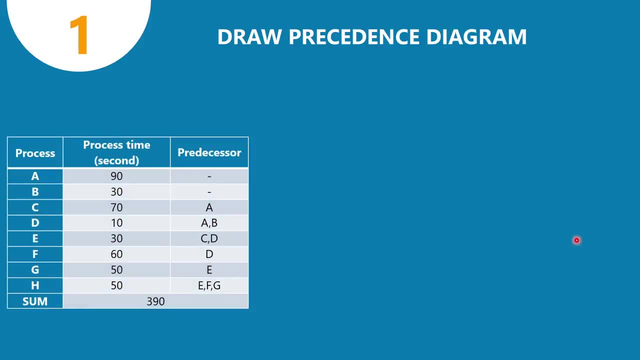 Let's begin with the first step: Draw the precedence diagram. Before we draw the precedence diagram, there are few things that we need to pay attention on. We have to make sure that there are some process which doesn't have any predecessor And it will be some process which doesn't have any predecessor. 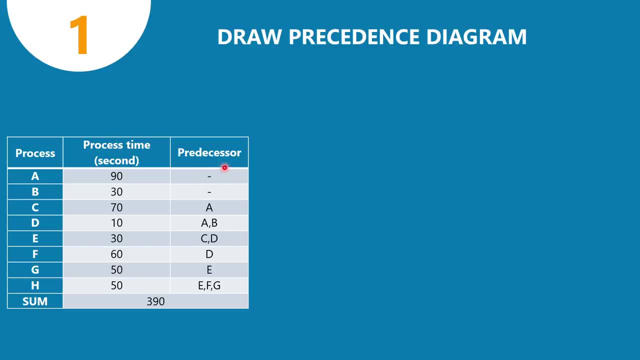 Predecessor means a process that requires particular process to be done before that process can be operate. For example, process C has predecessor process A, Which indicates that before we can begin the process C we have to make sure that the process A is being done. 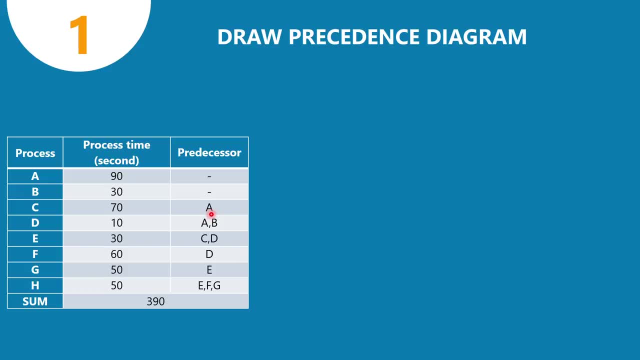 For example, if you want to make rice, Rice comes from wheat. Before you can make the rice, you have to make sure that you have wheat on your food storage, Otherwise you cannot make any rice. And let's begin, Because process A and B doesn't have any predecessor. we can begin from A and B. 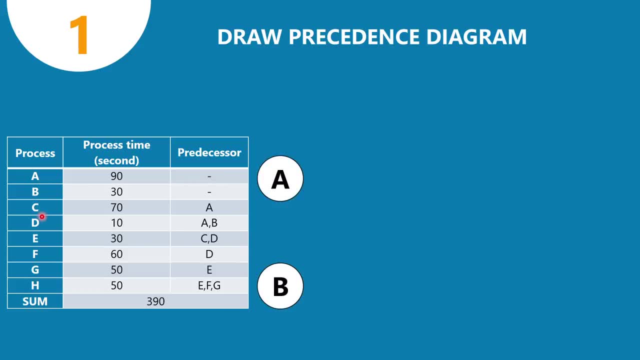 Thus we can proceed into the C process. It has predecessor A, Which means it can be like. this Indicates that it requires process A to be done before it can continue to process C. And then process D requires A and B, Which means that before we can begin process D, we have to make sure that A and B is already done. 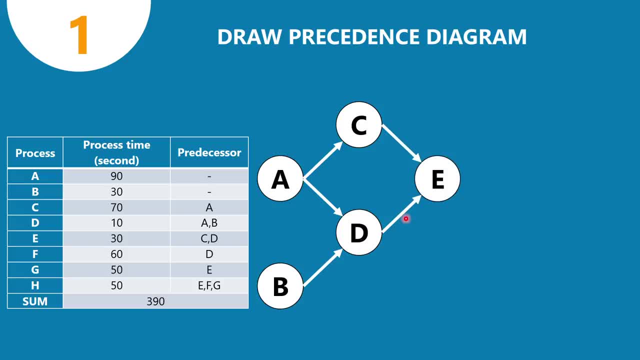 Otherwise it cannot be operate. And then process E requires C and D, Process F requires D, Process G requires E, And then process H requires E, F and G. After we're done making the precedence diagram, we can proceed into the second step. 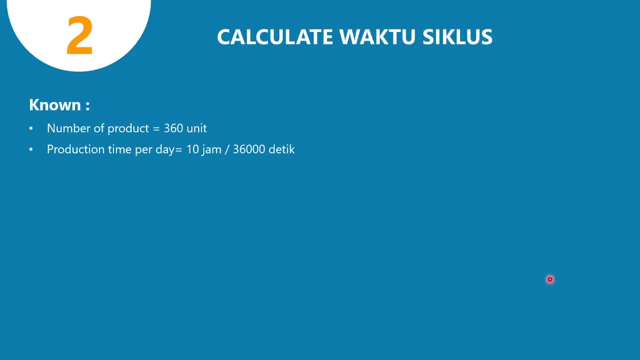 That is, calculate the cycle time. I'm sorry I haven't translated In the question paper. know that the number of products that are going to be produced is 260. And the production time per day is 10 hours or 36,000 seconds. 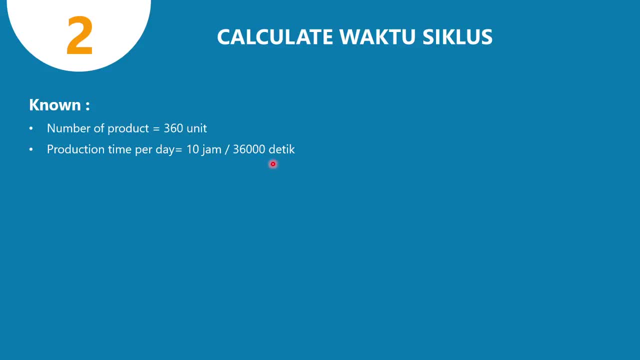 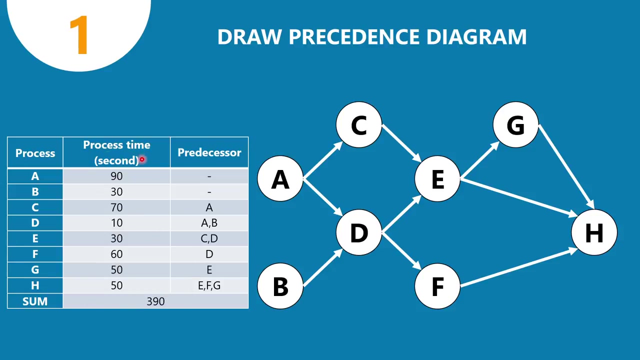 Why do we require to transform it into seconds? Because in this table it is known that The process time is in seconds. So if the question paper gives you some information in seconds, You can either change the second into hours, minutes or anything you want. 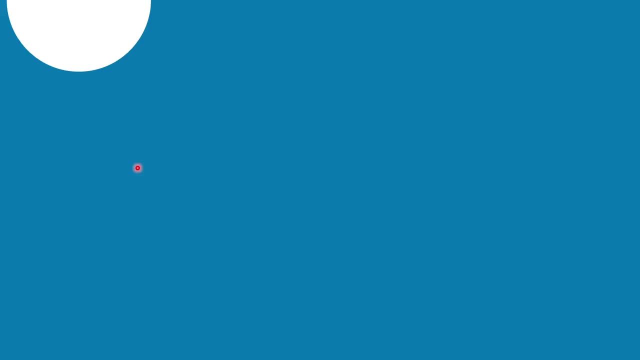 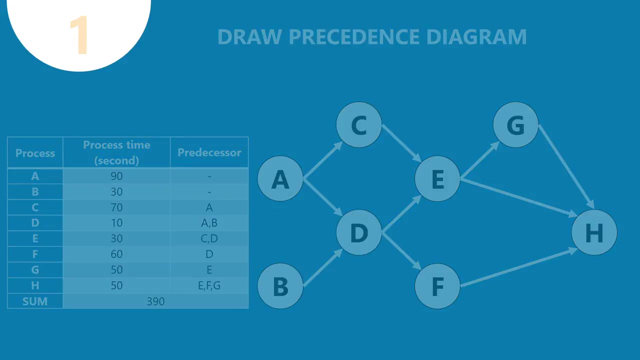 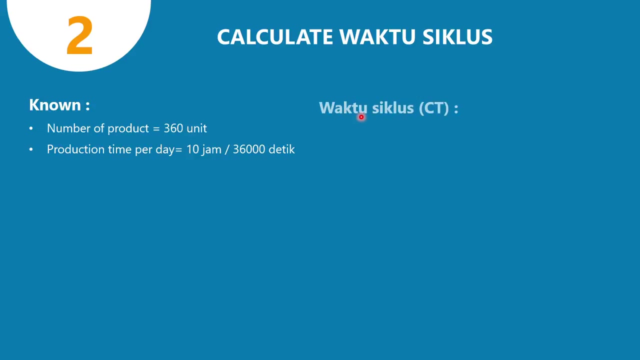 But it has to be the same. You can make it If this process time in this table is seconds. You cannot make this into hours, Otherwise it can't be divided. And then how to calculate the cycle time? It's by dividing the production time per day. 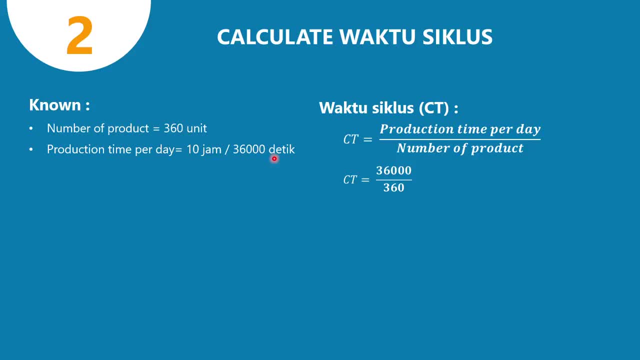 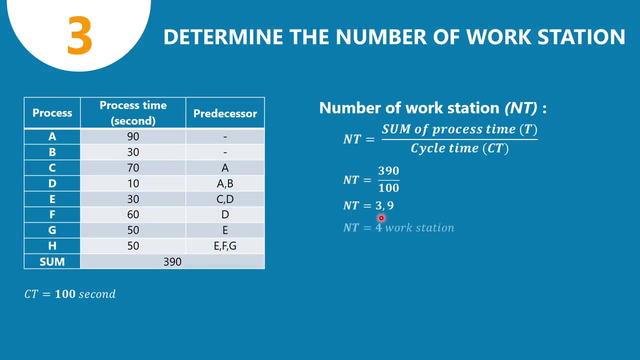 36,000.. I'm sorry, 36,000 seconds divided by 260.. And that is 100 seconds. So we can say that the cycle time is 100 seconds. And then we continue to the third step: Determine the number of workstations. 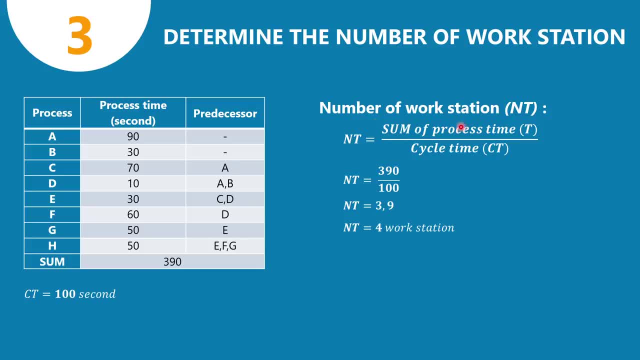 Alright. How to determine the number of workstations is by dividing the sum of process time, And this one process time: 60, 30,, 70,, 10,, 30,, 60,, 50,, 50. That is 292nd. 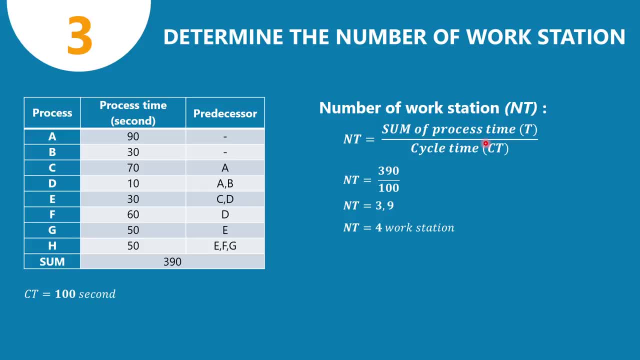 Divided by the cycle time Which we already been count before, That is 100 seconds. So 292nd divided by 100.. That is 3.9.. But we cannot make 3.9 workstations, do we? 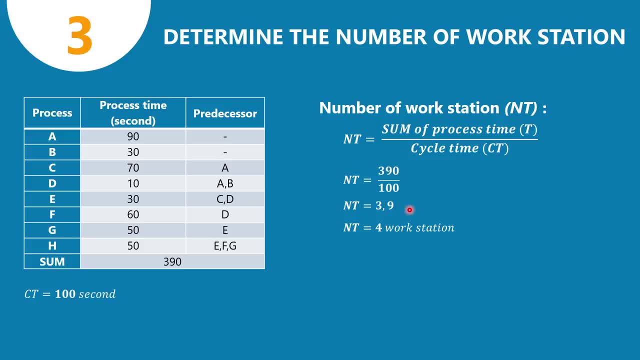 So we have to round up it into 4 workstations. Why do we need to round up instead of round down? Because if we round down, Round down the number of workstations, Round down the number of workstations into 3 workstations. 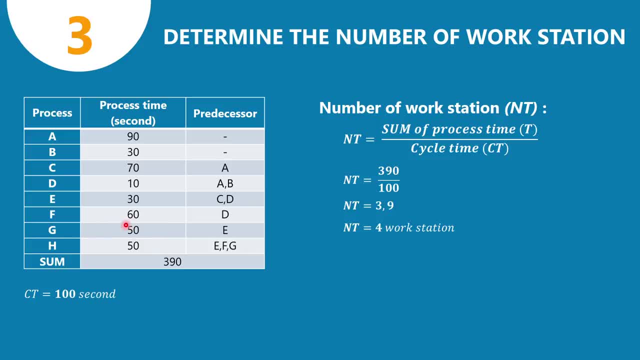 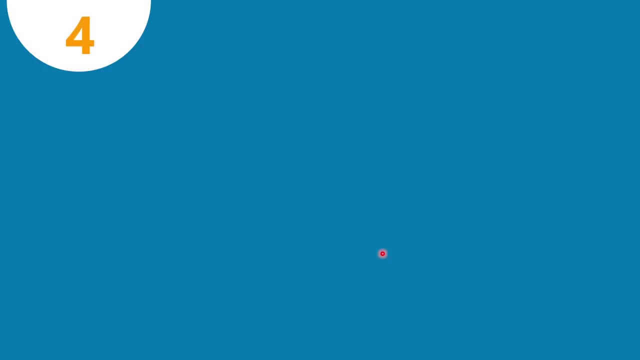 There will be some process which Will not be Processed, Because It just We Like the number of workstations, So we require to round up instead of Round down. Now we continue to the fourth, Into the fourth step. 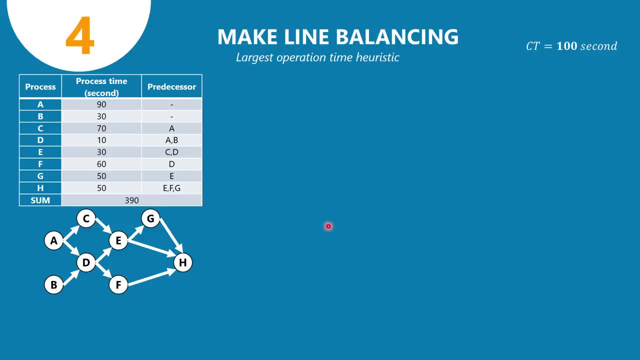 That is, make line balancing. Ahem, In the question paper It is clear that It is mentioned that we have to using The largest operation time: heuristic. What does it mean? Which means that In this process, When we try to make 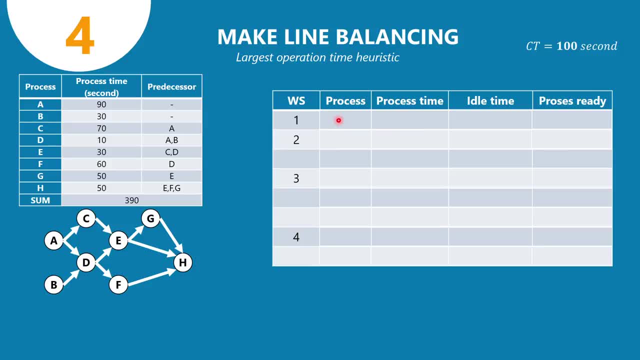 When we try to Determine which process to enter Which workstation, The process which has the largest operation time Become The priority. For example, let's begin From the workstation number 1.. There are A and B, Which doesn't have any predecessor. 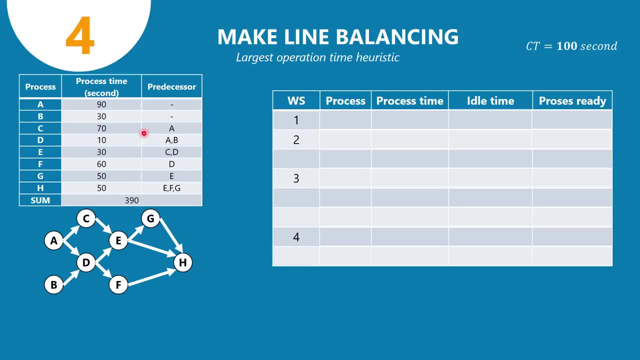 Which means in the first workstation We priority the A and B, But because we using the largest Operation time heuristic, We priority which process That has the Largest process time. In this table it is clear that A Has the largest. 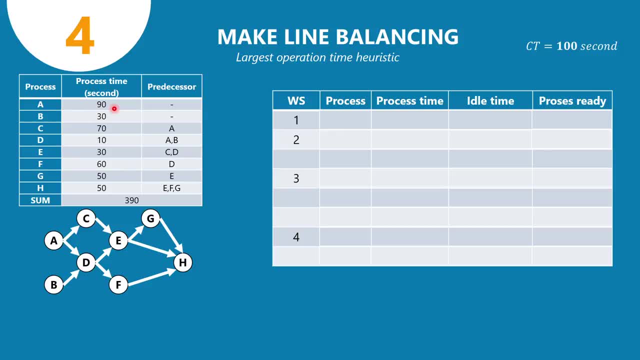 Operation time Of B. It's 90 seconds Out of 30.. So we chose the process A Instead of B, Which Has 90.. 90 process time And idle time. How do we get idle time? 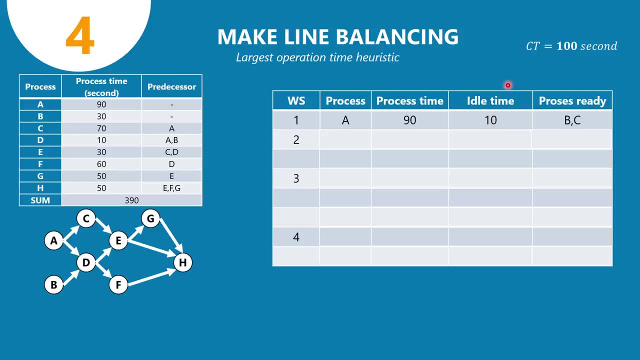 Idle time. We can. We can get idle time by Subtract it, Subtract the 100 seconds. I mean minus, I'm sorry, By By subtract the 100 seconds With the 90 seconds, So we can get the idle time. 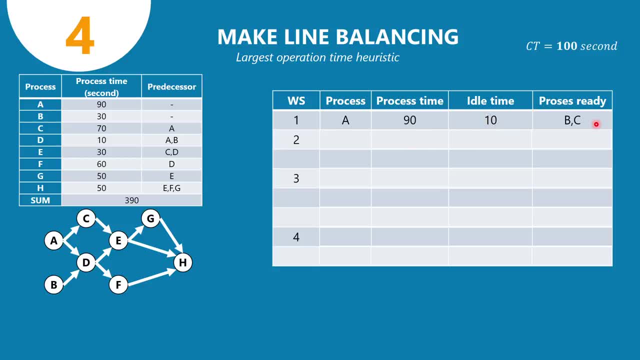 10 seconds And the process ready. here There are B and C, Which means that The process that Can be chose In the next step Is B and C. Why we cannot choose D? Because in order, In order to chose D, 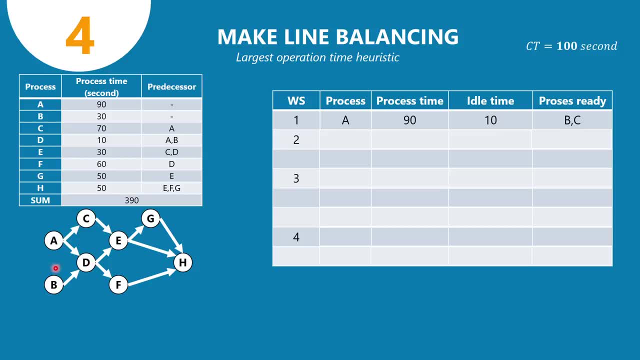 For example, we have to finish Process B first, Because process B Is have Not yet Not yet been chosen. We cannot chose D. We have to finish B first Before we can begin, Before we can begin the process D. 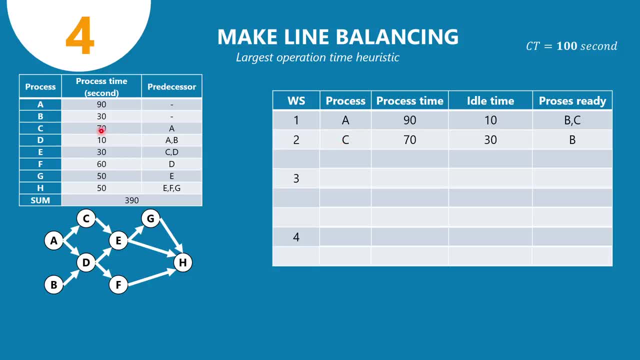 Therefore We chose the process C, Because it has the largest operation time, Instead of B. B only have 30.. C have 70. So we chose C And we have the idle time: 30.. By subtract 100 with 70.. 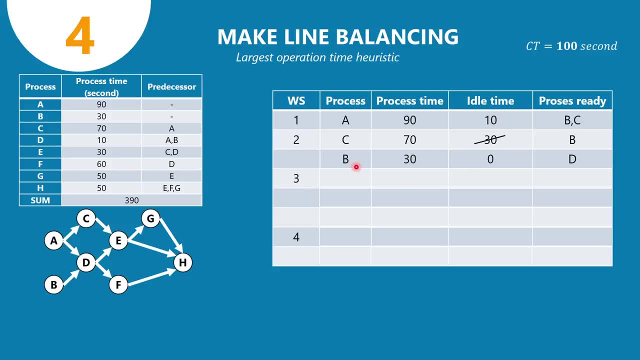 And the process ready. Process B. So we chose D And we chose B. With 30 second process time And the idle time It became 0. Because the idle time In the previous step In the C process. 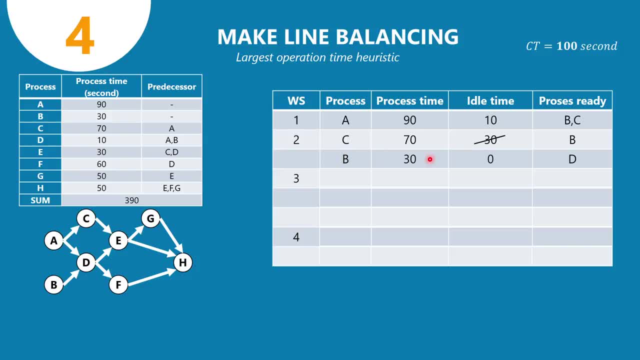 Is already been cover in Process B, So we Erase the idle time over here And the idle time On the workstation 2. Is already 0. Because the idle time Is already been 0. So we can. 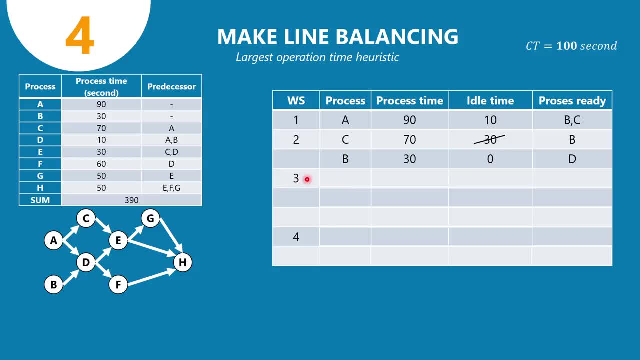 Proceed into the next workstation. Alright, Because the process ready is. only step Is only process D. We chose the process D With 10 second of operation time, Then we have 90 second of idle time, Then we have E and IF. 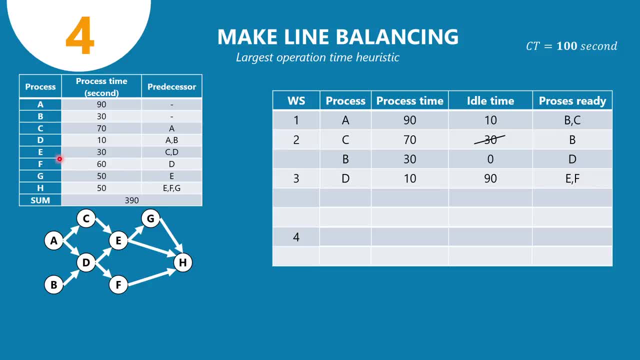 As the process ready E and IF F has the Has the largest operation time Over E, So we chose F With 60 process time And the idle time became 30. And the process ready is E, Then we chose E. 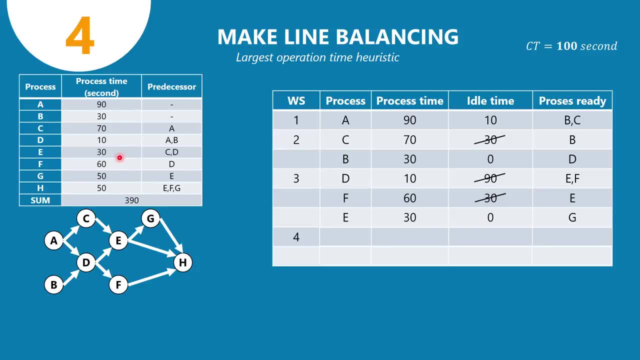 With 30 second of process time In this table. Then the idle time Became 0 again. After the idle time is 0. We can proceed into the next workstation In the workstation number 4.. We input the process G. 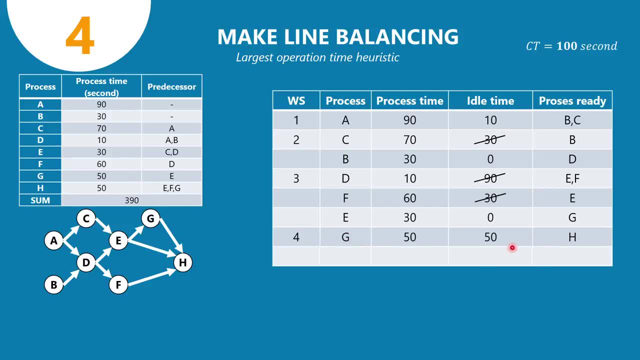 With 50 process time. Then we can proceed Into the process H, Because E, F and G Is already been Input in here. Then we can go into the Process H With 50 second of process time Out of 10, 0.. 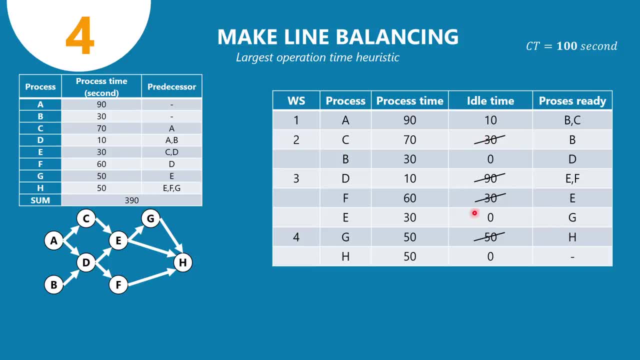 So when we look at the table Over here, We can say that the idle time, The total idle time Of our production line Is only 10 second. This information is important When we Determine the efficiency. Alright, We already. 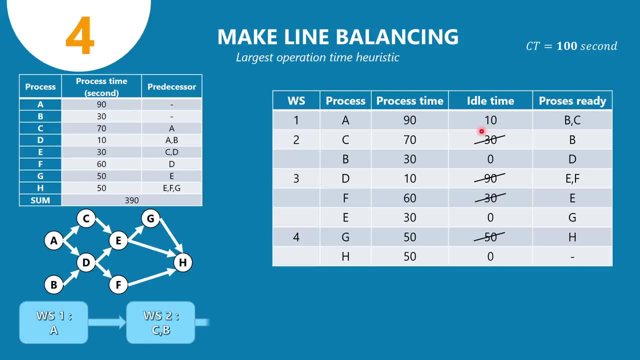 Know. These are the Production line That we going to using In the workstation number 1.. There are Process A In the workstation number 2.. There are C and B Workstation 3.. There are D, F and E. 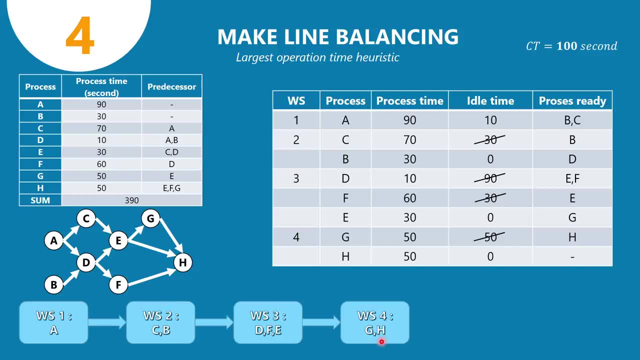 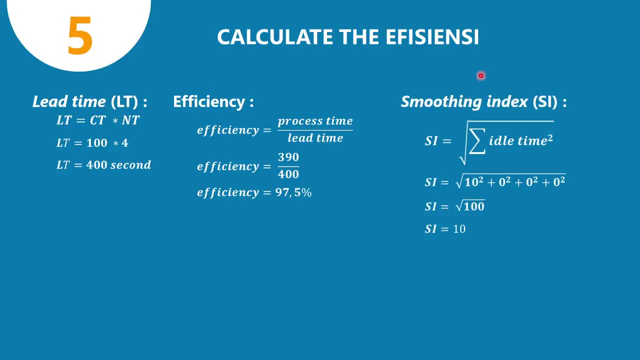 In the workstation 4.. There are G and H. It's time to determine Efficiency. I'm sorry, It's typo again. First we can measure the Lid time. Lid time, which, Uh, Whole time that required to produce. 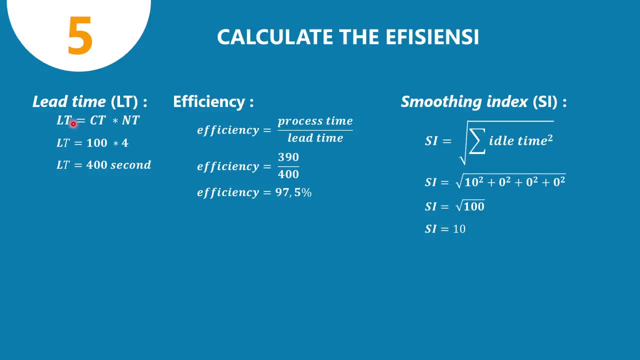 One product. Yeah, One product. I mean The amount of time which Been through by one product, Lid time. We can measure the time by Calculate the Cycle time Multiplied by Number of workstation. We have 100 cycle time and 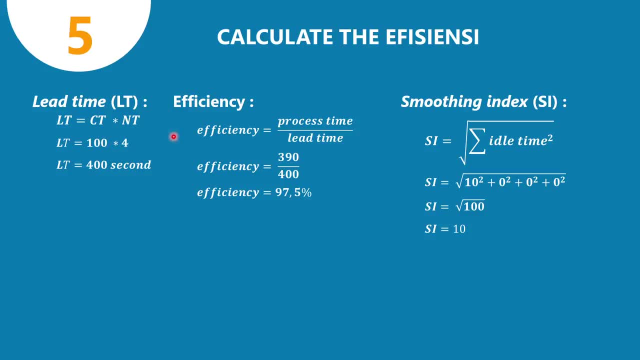 4 workstation. Therefore Lid time is 400 second And the efficiency We can divide the process time, Which is 290.. Divide by Lid time 400.. We can get Efficiency 97.5% And smoothing index. 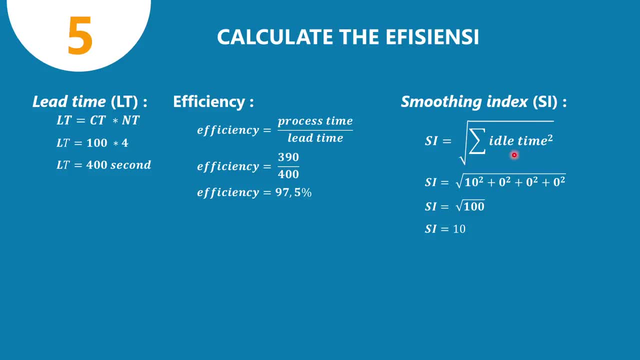 Smoothing index Is the square Total of idle time. But Um, It should be. It should be square first, Multiplied by idle time again, Because in this table We only have 10 second of idle time. We just